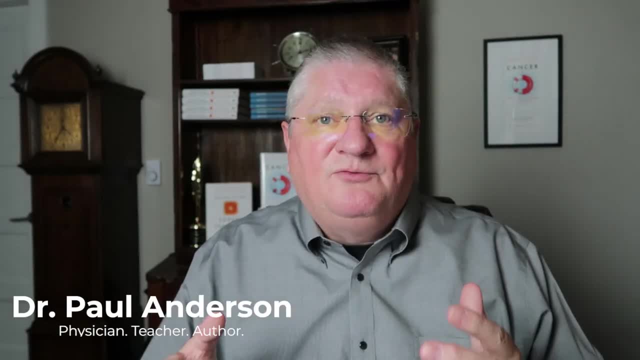 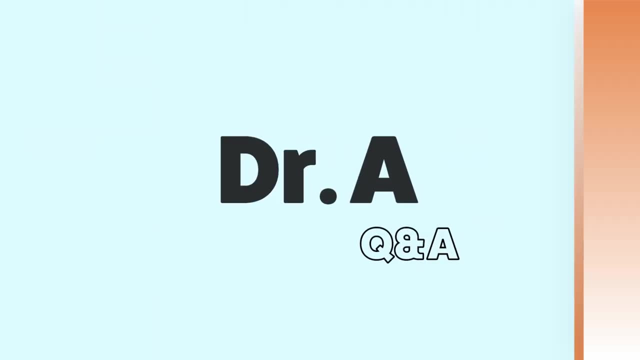 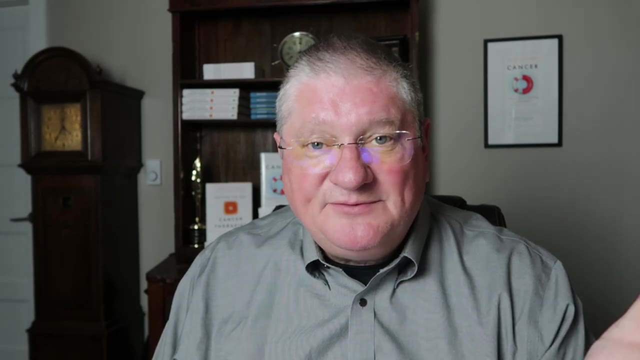 In this paper. when they say lead and cadmium, we've now got proof that they're not just associated. These are definitely bad for you and bad for your cardiovascular system. So you know, heavy metals are probably bad for humans. but how specifically In the Journal? 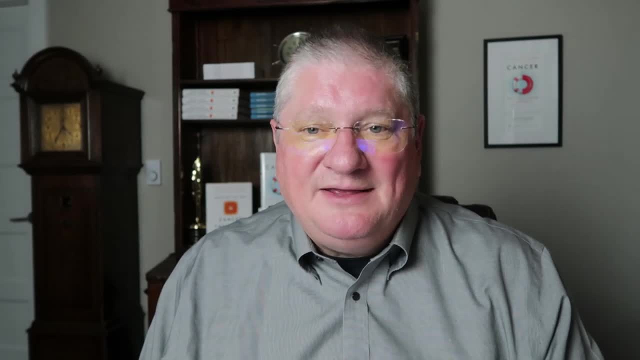 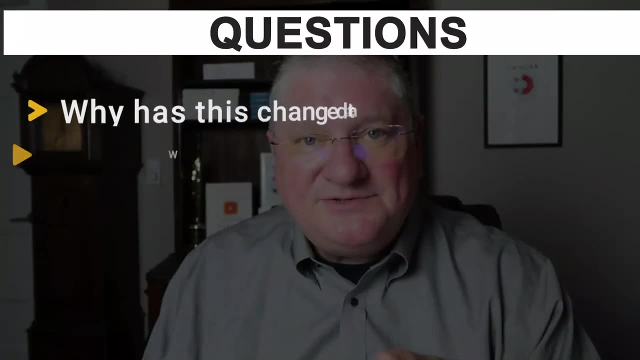 of the American Heart Association, there's a paper about lead and cadmium, and lead and cadmium have been shown to be cardiovascular risk factors. Why has this changed the game? Why is this important? What does it tell us about what we used to think and what's it mean for your health? Well, I'm Dr. 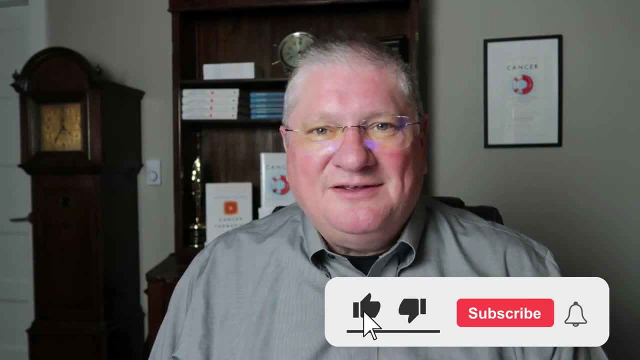 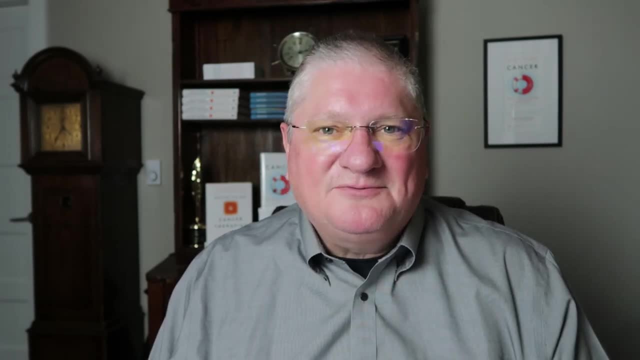 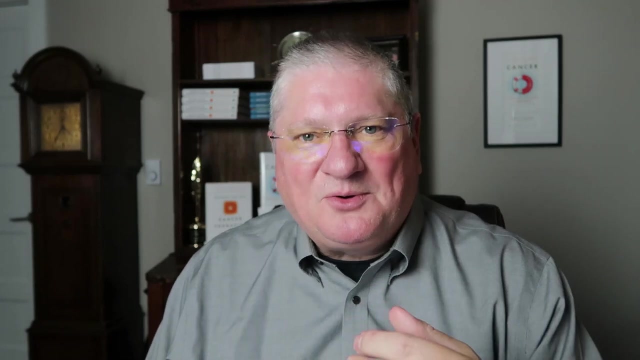 Ray, I answer questions here on this channel. I've been in the world of medicine as an educator, writer, researcher and physician for the last three decades and it's a lot of fun answering questions that get sent in. This is a little bit more about a paper and I've gotten this question. 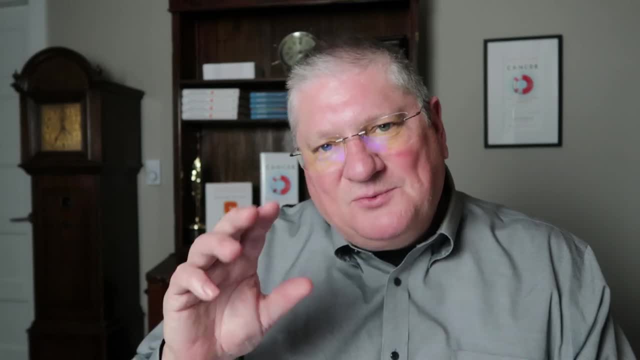 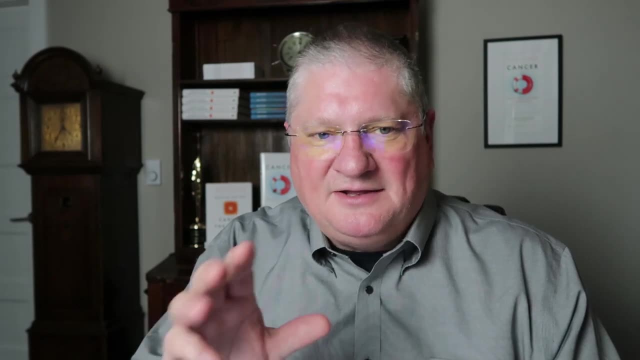 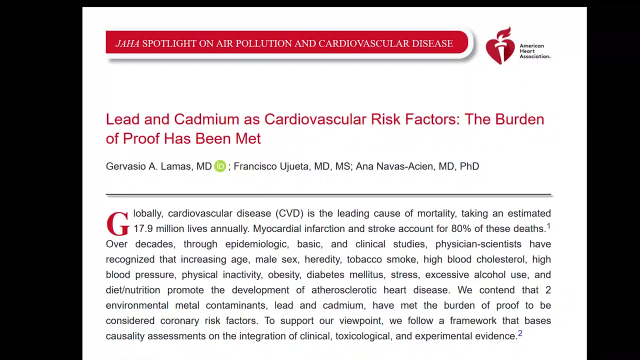 generally, So I just put them together into a question. If you want to go, look at this paper in the Journal of the American Heart Association, this is Lamas et al- L-A-M-A-S is the doctor's name, Et al means a bunch of other people wrote- and it's called Lead and Cadmium as Cardiovascular. 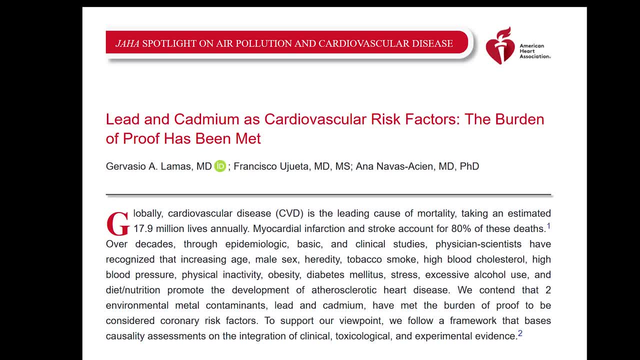 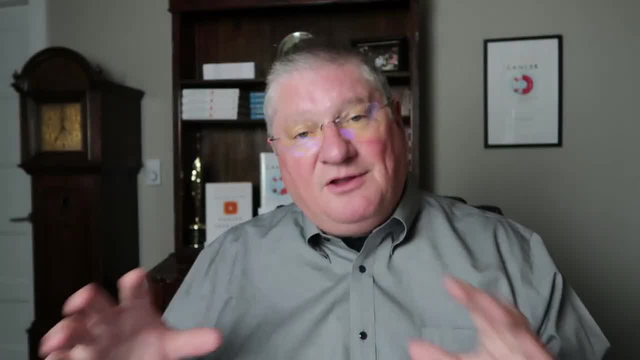 Risk Factors. The Burden of Proof Has Been Met, and that is Journal of the American Heart Association 2021.. So it's a recent paper. but what's this burden of proof has been met Well, for a long, long time. 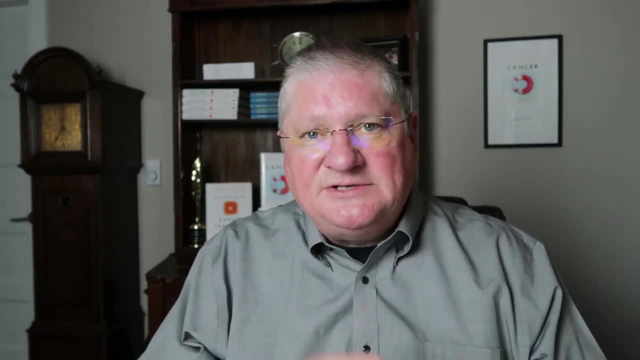 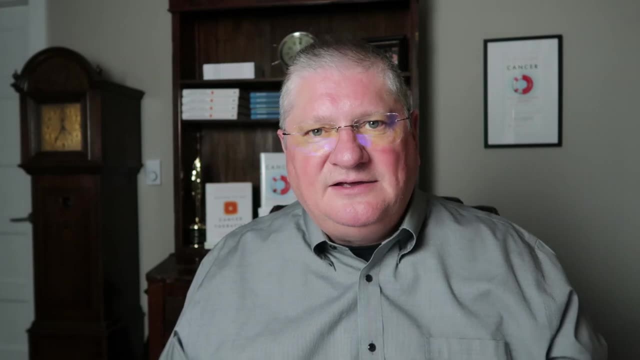 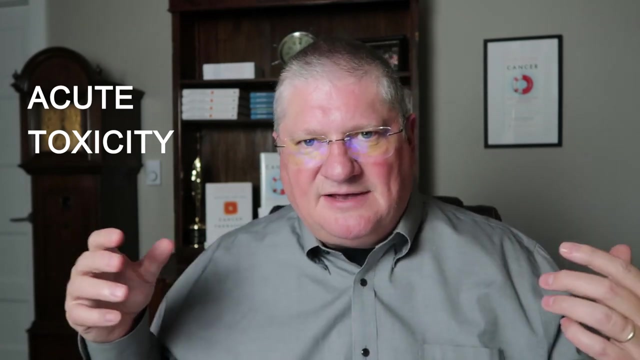 Because I teach about heavy metal toxicology et cetera. we would teach that there's these associations between cadmium and these diseases and arsenic and these problems. Now there's obviously acute toxicity. There are cases such as I've testified on in other forums, not on you. 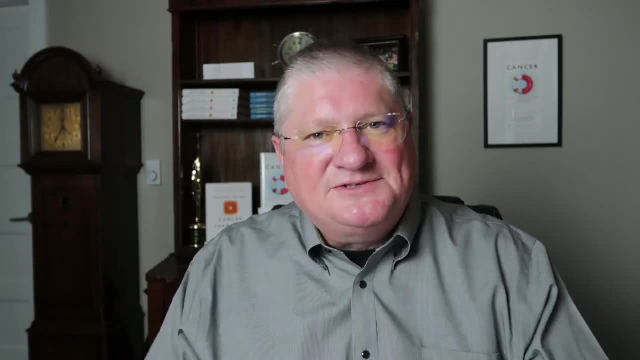 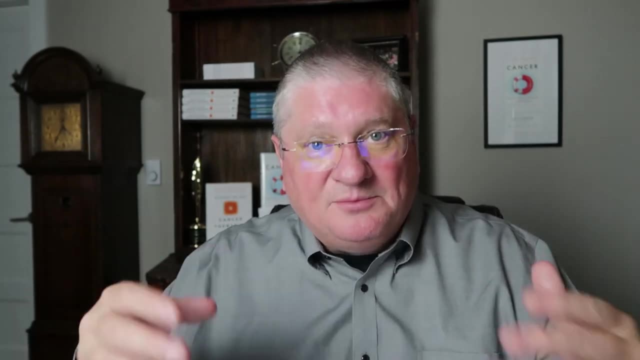 I don't testify on YouTube, just tell you stories. I've testified about cases of acute arsenic poisoning where someone tried to kill a bunch of people and killed one. Thankfully other 15 were able to be treated and they lived. Obviously there's acute poisoning. 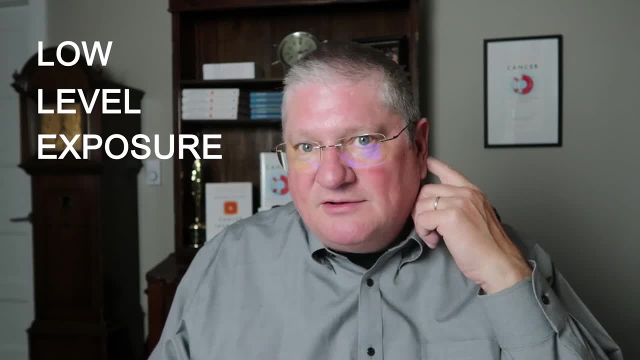 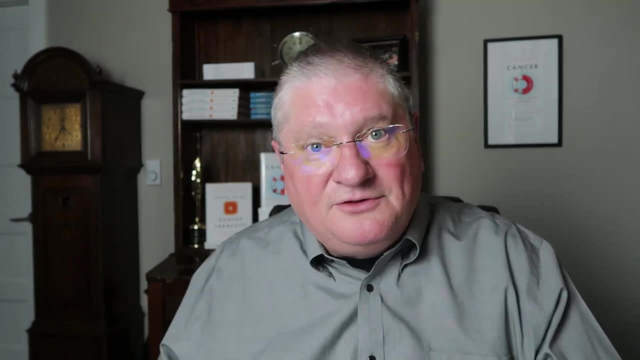 but what about low-level exposure? My colleague and friend, the late Dr Walter Kranian, used to be very, very big into researching low-level exposure and its effect on your health, and that wore off on me because we would teach together. When they say, the burden of proof has. 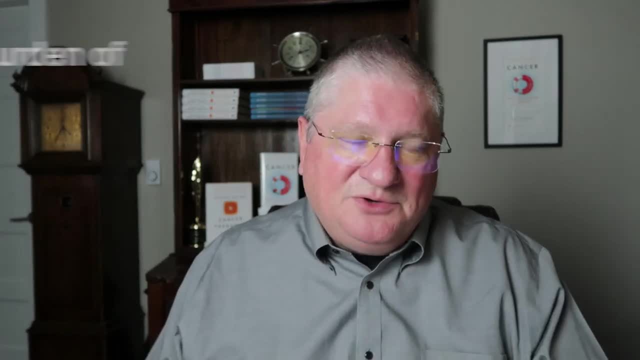 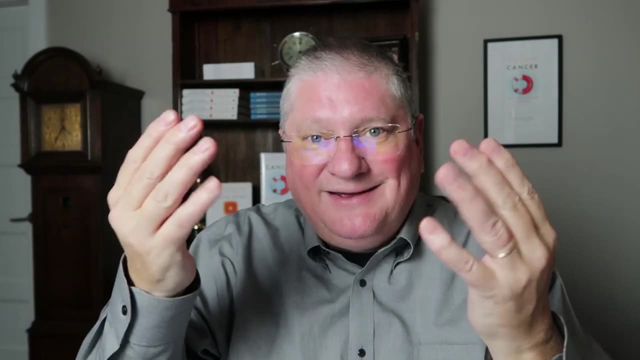 been met. what they're saying in the Journal of the American Heart Association is: we've thought for a long time these things are bad for you. They appear associated with bad heart disease. We're not sure what they mean, but we're not sure how we see why. I think this is opening. 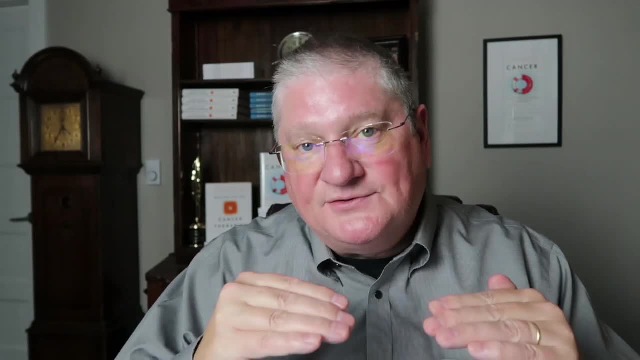 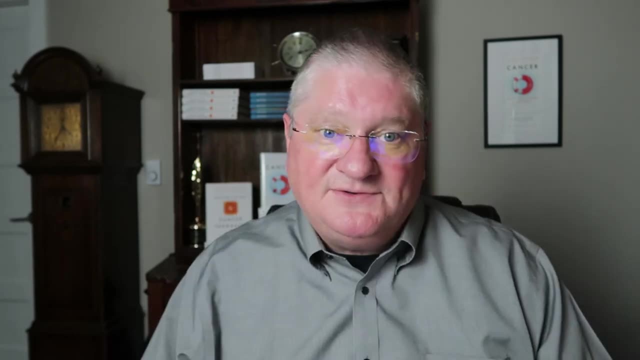 the door to an understanding that non-deadly poisoning levels of metals- environmental toxin levels of metals- are still important to look at. as far as your health goes, It's still important to minimize because obviously, if just these two metals do this, imagine what others that we 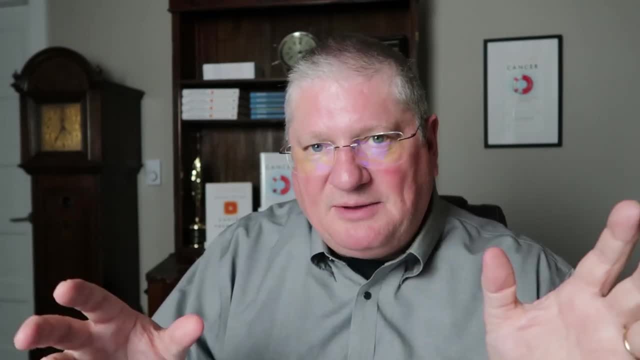 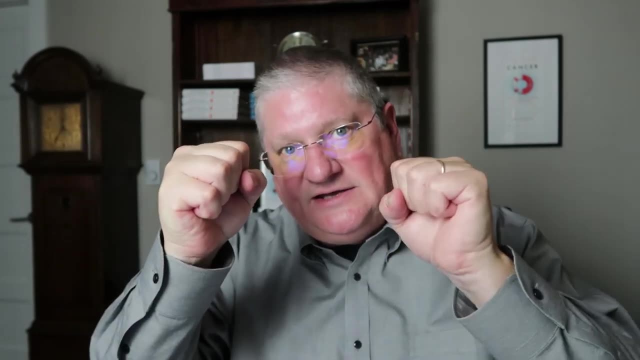 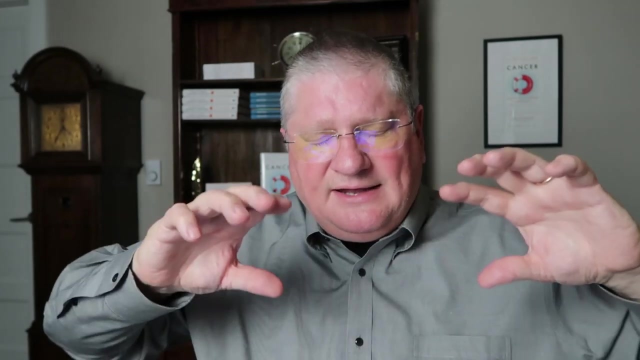 haven't talked about, like arsenic and other things, do I want to go through? you can read the paper if you want to. Why, would they say? the burden of proof is met that cardiac disease and these metals can be associated with each other. but what do they do? Well, in both cases they get involved where other 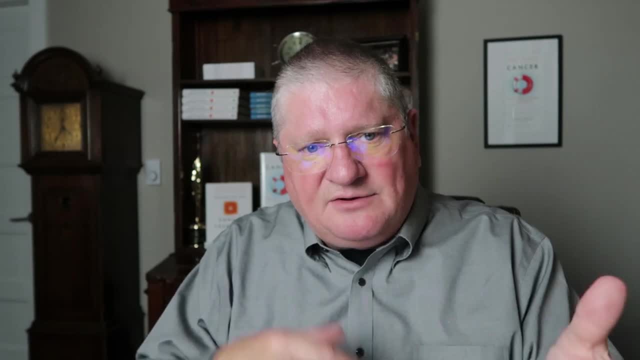 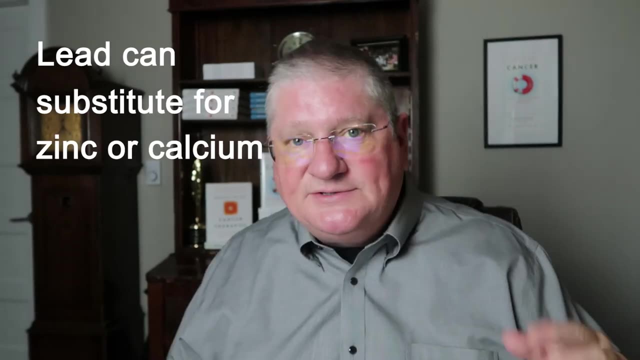 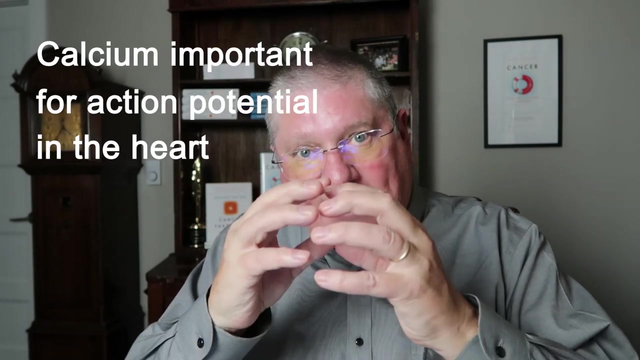 minerals should be so. they substitute Lead or cadmium can substitute for other things. For example, lead will substitute for zinc or calcium. Now, zinc is incredibly important in a lot of things. It's actually making your action potential, the electrical charge in your heart. 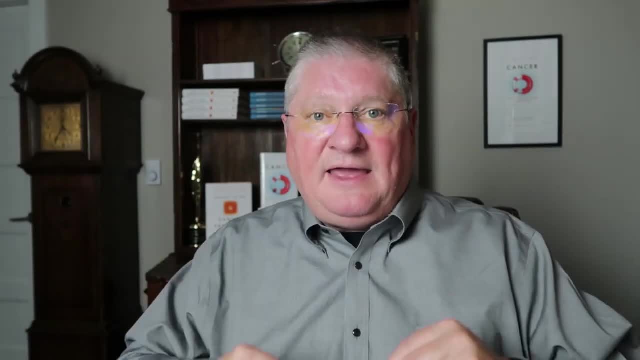 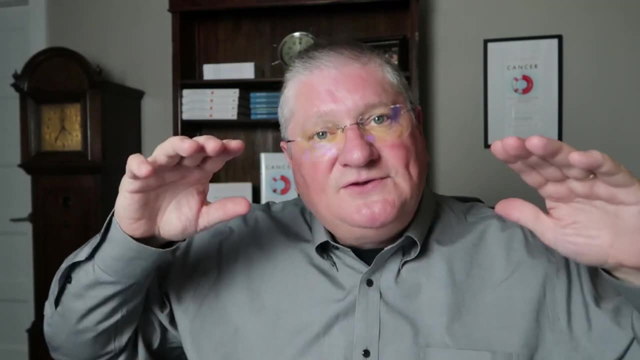 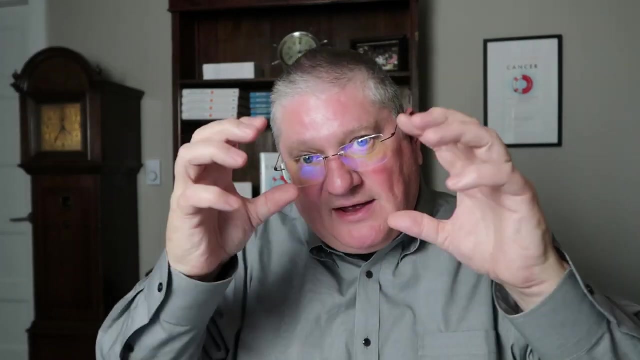 muscle operate. So these are pretty big deals, right? They lower levels of antioxidants, both of them cadmium and zinc. Both of them decrease nitric oxide. So you've heard of nitric oxide That helps the blood vessels relax. If we have low nitric oxide, we have tight blood vessels. We 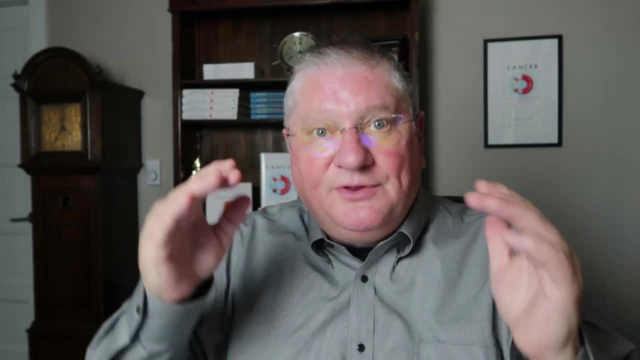 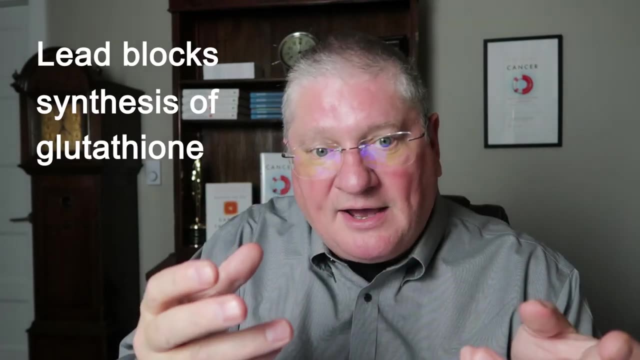 have higher blood pressure. Other problems go on, Both of them lower nitric oxide. Lead actually blocks the synthesis of glutathione, which is one of your primary antioxidants, And while it does that, it decreases another primary antioxidant called superoxide dismutase. 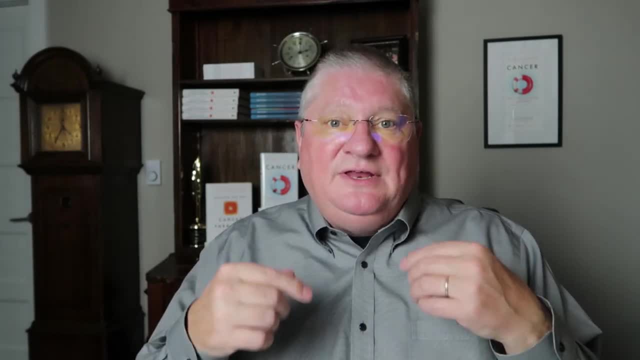 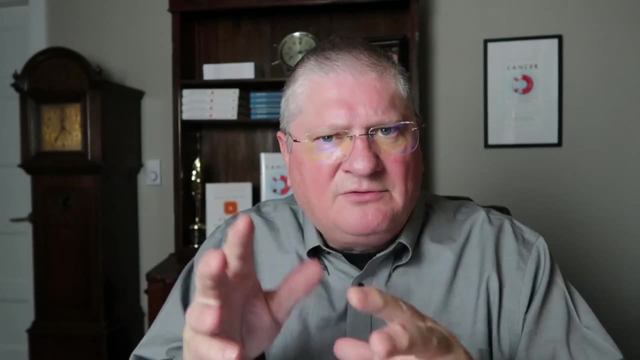 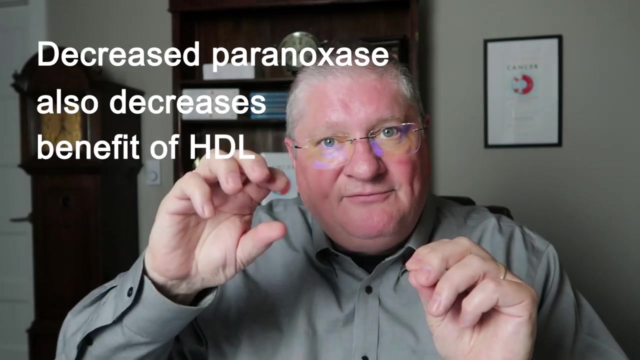 That's bad enough on its own, but it also decreases paranoxase activity. So that's a long word, but what does that do? Why would we be decreasing that? It'd be bad for my heart. Well, paranoxase: when you decrease it, it decreases the benefit. your HDL. 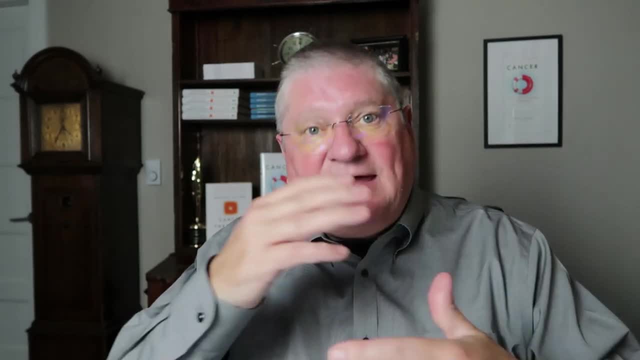 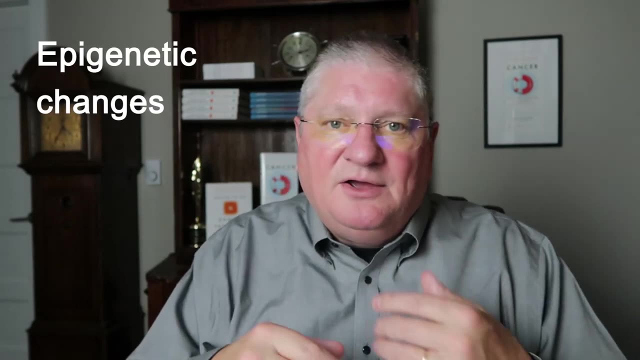 the good cholesterol gives you. So when you have this effect, your HDL is not as good for you anymore. The other thing it does, as both do, is epigenetic changes. So remember we talked about genetics and how that's the code, but epigenetics are what affects the code. Heavy metals are huge.